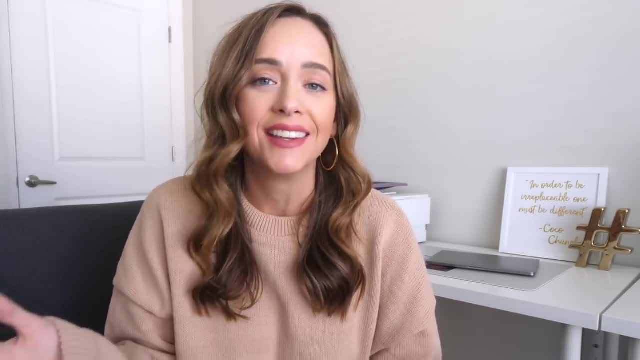 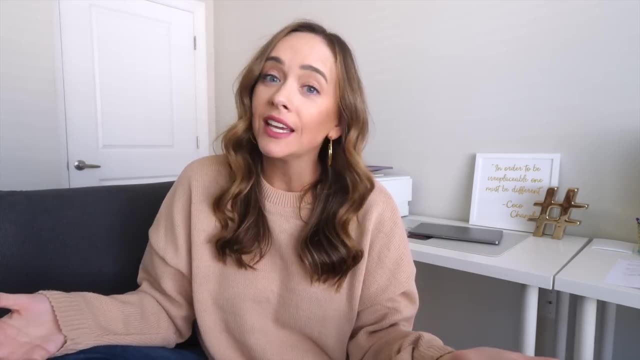 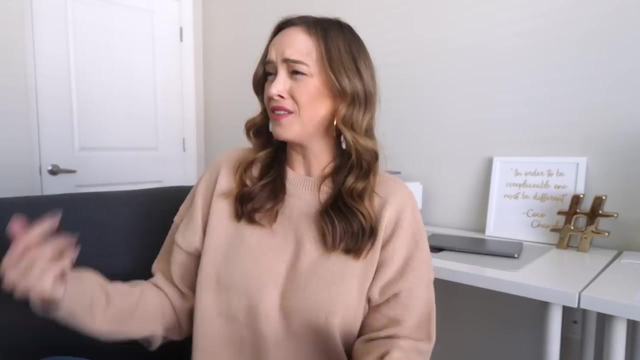 has come where everyone's very excited. What's Amy got to say about managing your time as a parent when you are dealing with the dynamics of taking care of your kid and also getting work done and getting things done and making sure you survive? And, oh my God, are we surviving? I don't know. 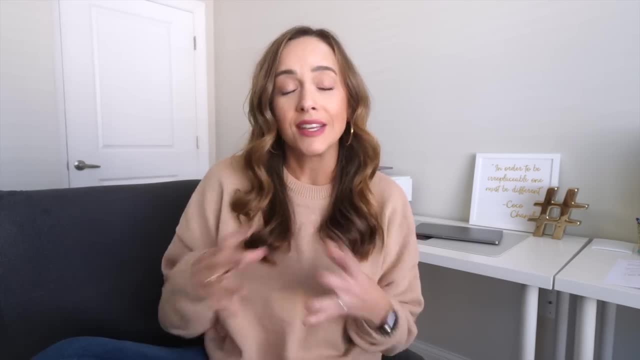 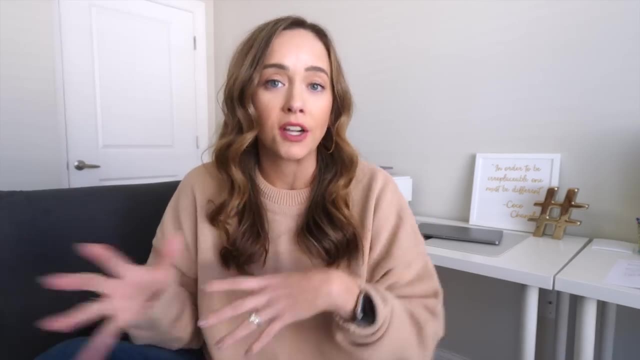 A lot of things that I have talked about in the past. when it comes to managing your time, really work across the board, Whether you're a parent, whether you're not a parent, whether you're a college student, whether you're a, I don't know. 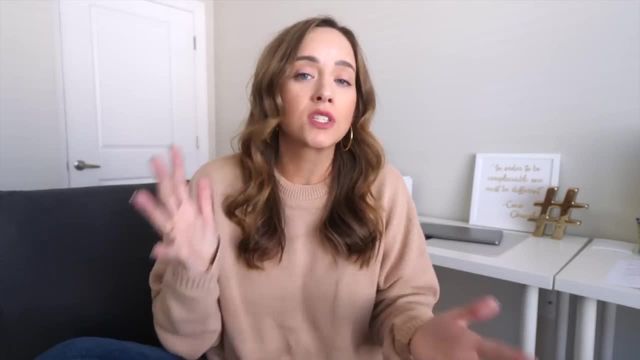 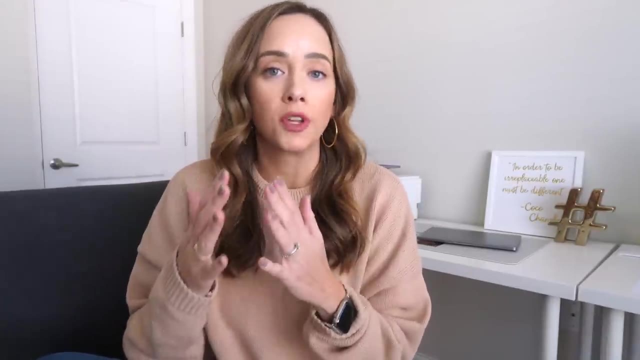 Anybody, literally anybody. But it only works when you believe in it. And when you believe in something, you give it so much focus Everything really just is fueled by that. When you do not have focus, it's not going to work. When you do not have focus on whether or not a tactic's going, 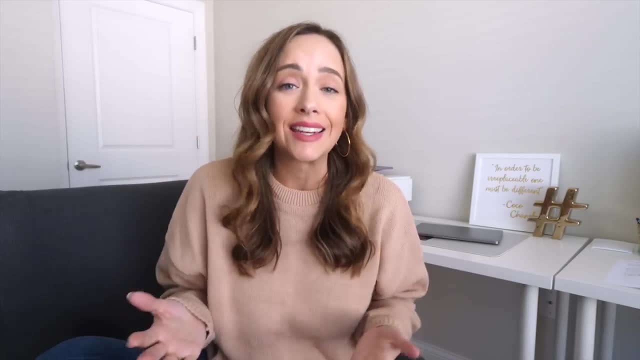 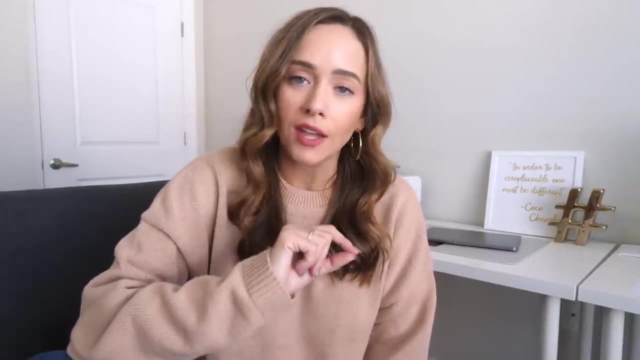 to work for you. it's not going to work If you do not have focus on the task. it's not going to get fully done, or done to the best of your ability. But what I would add is probably one of the biggest challenges that I've had in my life. 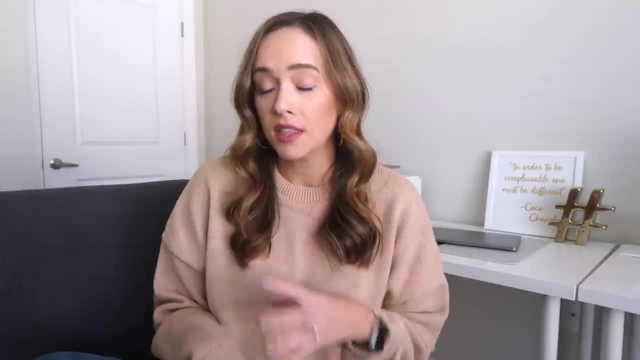 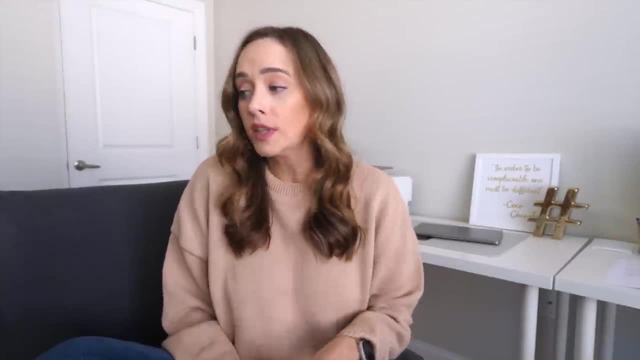 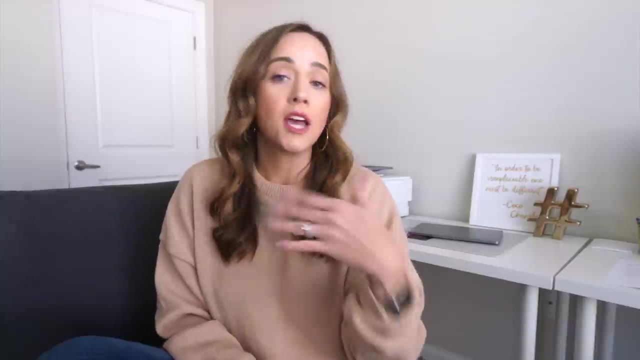 So whether it's like your time batching, which actually really interestingly, I just did a video with Morning Brew. If you haven't heard of Morning Brew, they have a killer newsletter telling you all of the wonderful things that are going on in the world, but in a way, that's. 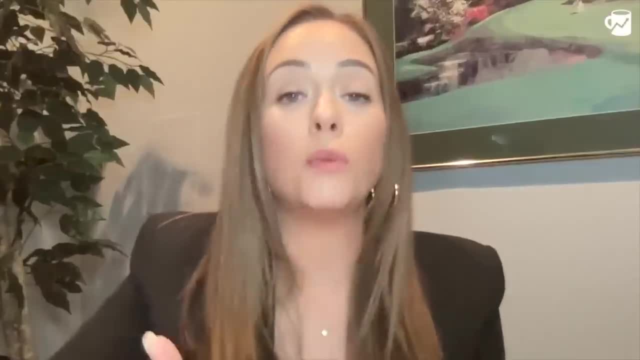 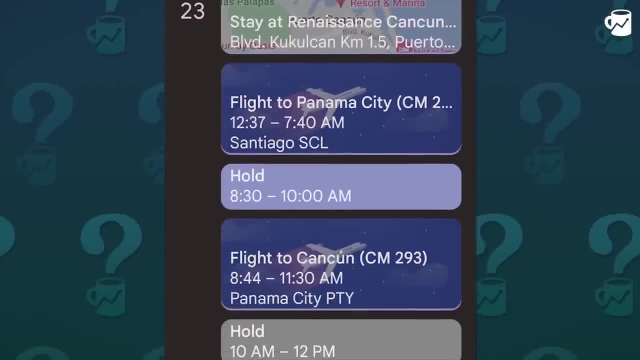 actually kind of fun And they wanted me to challenge their team on how to be a bit more productive with some ideas that I have, And one of the things that went over really well was time batching- Just the concept of blocking time on your calendar for like tasks, An example. 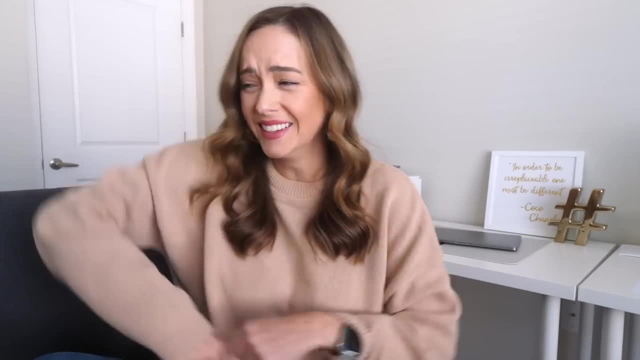 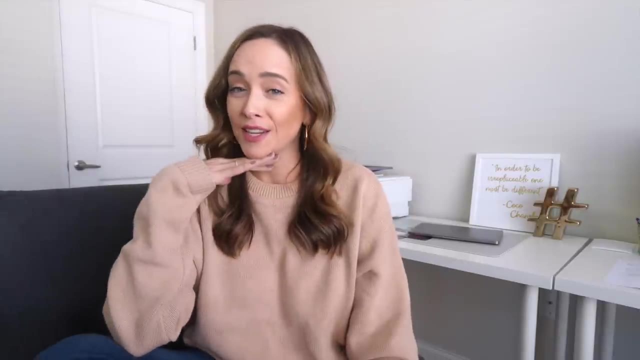 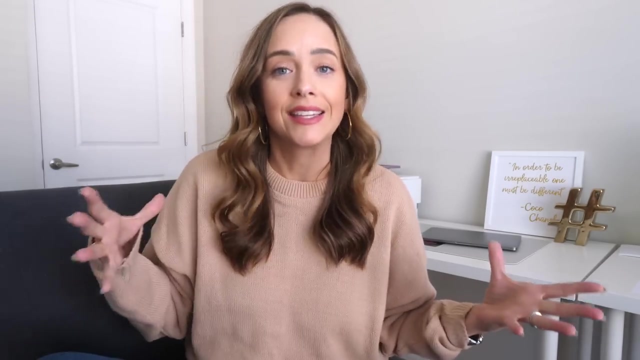 currently, in this moment in time, I am borrowing. I'm not joking, I'm borrowing someone's home office and passing it off as mine And as I sit here, I'm doing a few filming things I got to get done. because I'm going to batch like tasks, I'm going to have my makeup on. 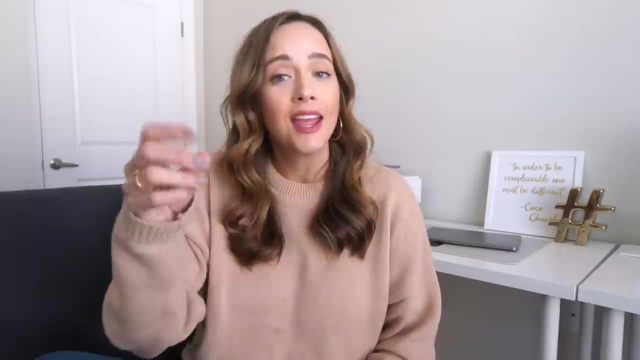 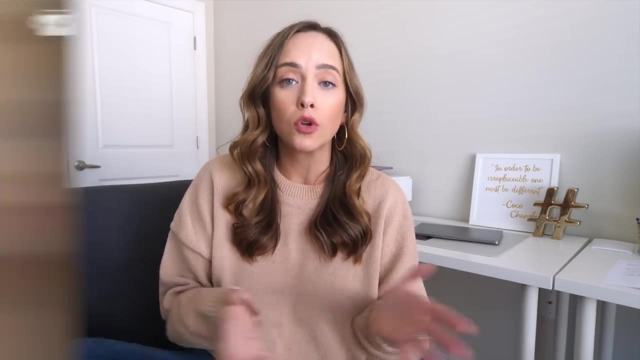 and I'm going to use it up to the best of my ability. I've been fully caffeinated camera's going, so we're going to do as much as we can in this moment. Time batching like tasks went over really well with that group. 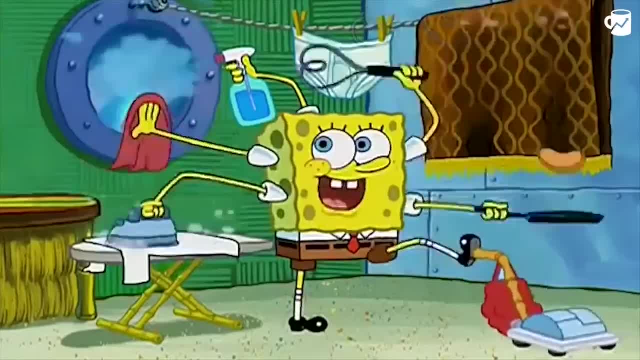 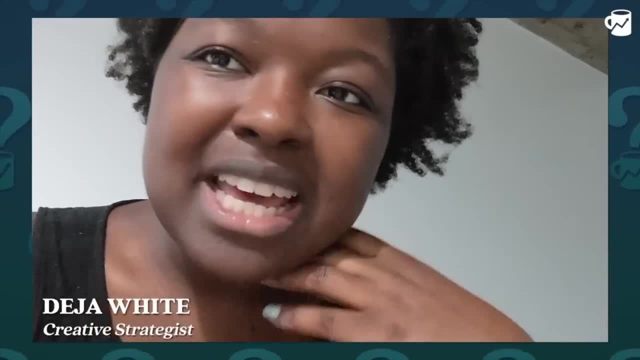 Some batching today. So me and the roommates actually batched all of our chores and cleaned the entire apartment. The entire apartment: spick and span, great as new. Something else that I did today was put working blocks on my calendar. It's one thing to have like. 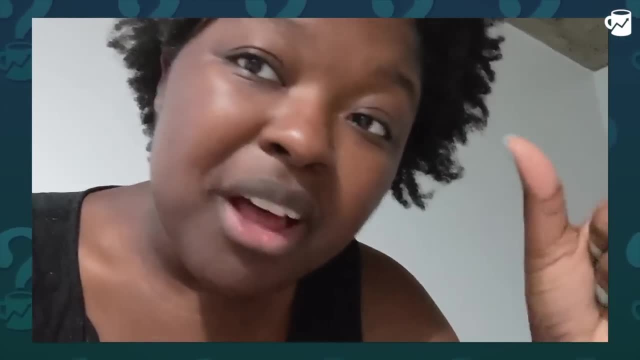 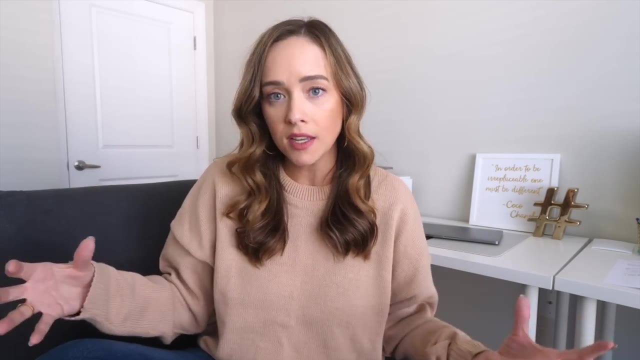 my meeting blocks, but it's another to put actual working blocks on my calendar. So I'm proud of myself. I'm making this happen, I'm making this happen, I'm making this happen, I'm making this work, And it's because you can get a lot more done when you're doing a lot of the same thing. 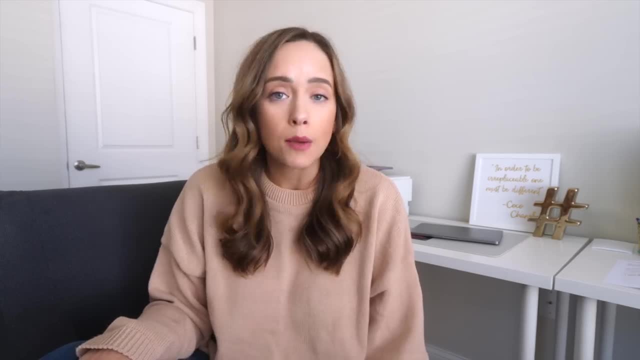 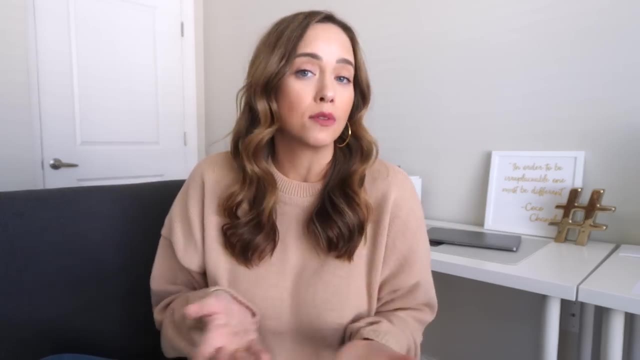 back to back because you're in a flow. So time batching, that's just one example. Calendar blocking, that's one example. Using a focus timer, listening to brain stimulating music or sounds that helps you focus- There are so many different things that you can do. 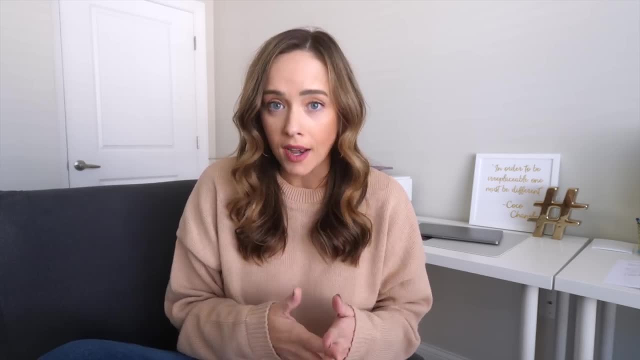 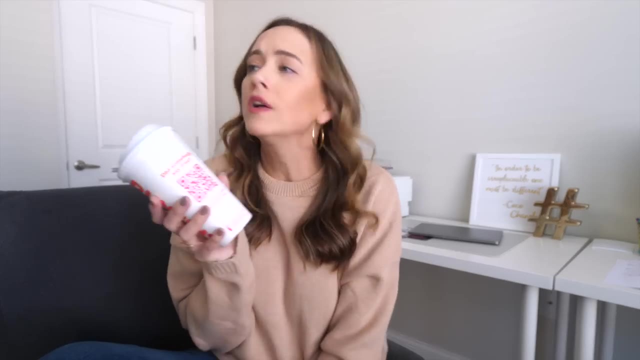 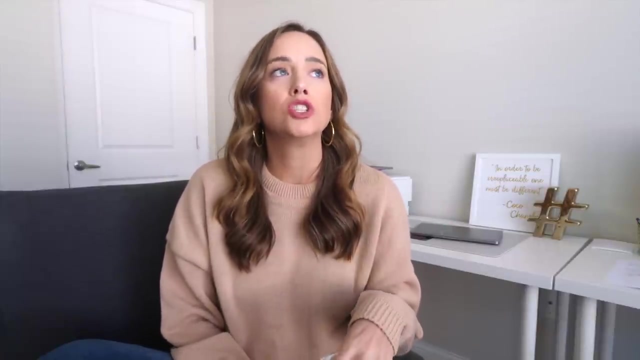 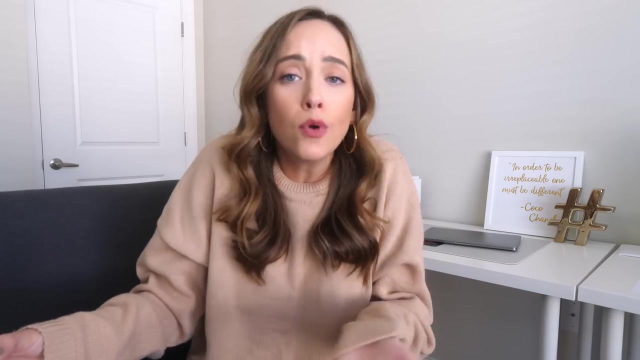 but they're so much more successful when you ask for help. I don't want to. I don't want to. Okay, Asking for help has been one of the most challenging things for me throughout my life. in so many ways, I don't know what it is, I really I feel like it has a lot to. 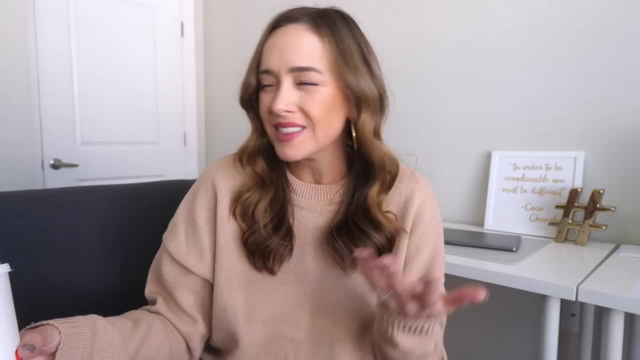 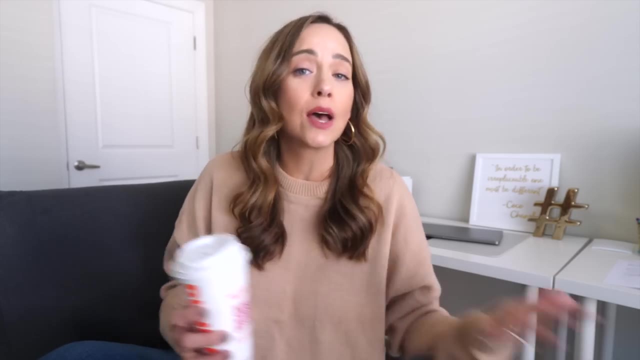 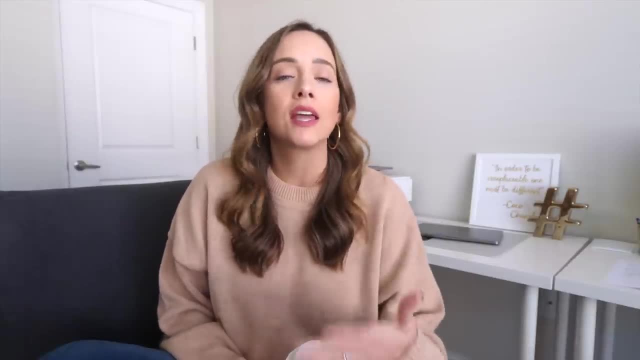 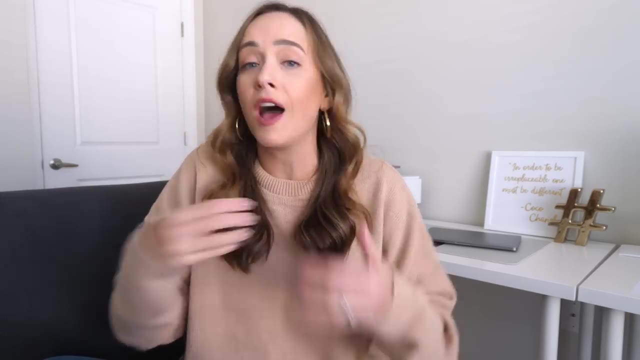 the best of my ability and then see where we go from there. And I realized that that is not all asking help really is. And as much as I've talked about everybody getting better at asking for help on this channel, I've always been coaching myself on that at the exact same time. It's not just 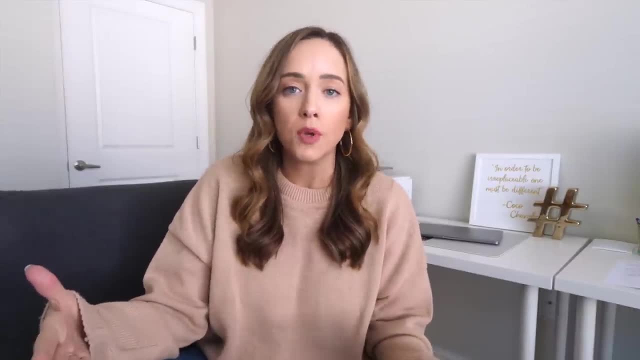 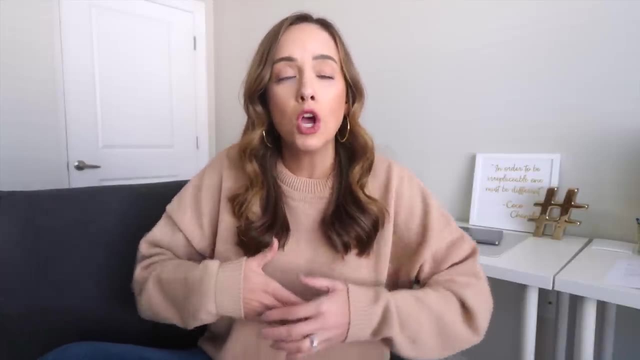 about the fact that you can prove you're capable of doing something. You can also prove to yourself that you're capable of doing something, but you're capable of asking somebody to help you with it as well. So you do not get yourself into the. 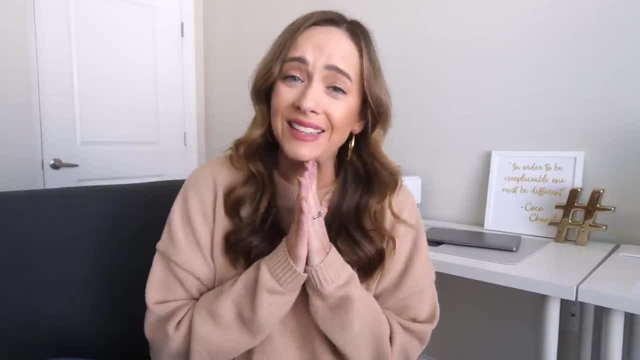 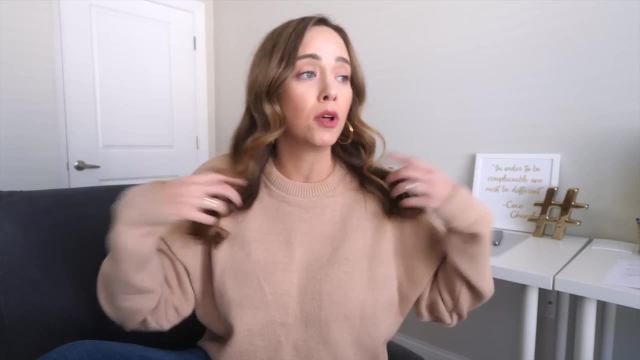 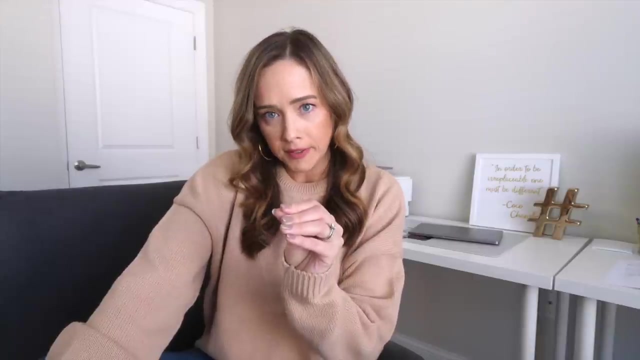 type a stress ball of a human being that I happen to be. So asking for help has always been really challenging for me because, again, I don't want to put people out. I am fully capable and fully independent. I am fully resourceful. Love that for me, Love that, But then a human that I pushed out. 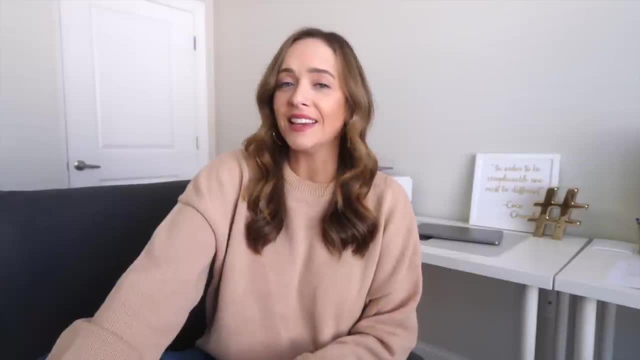 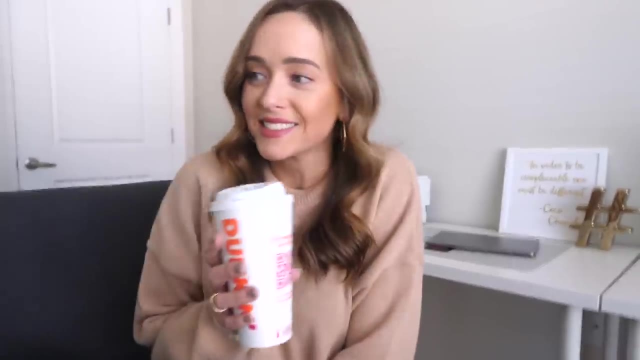 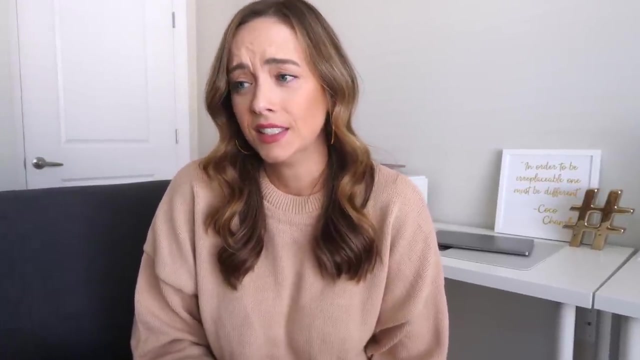 of my body came to this earth. Silly silly Amy. She thought I'm just adding more humans to the earth. I can still do all the things that I say I can do Turns out. yes, I can, but only if I'm a. 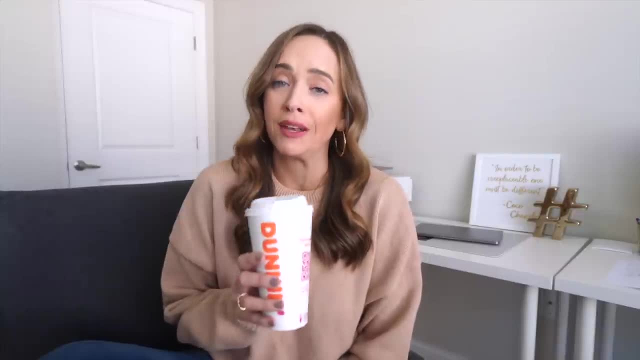 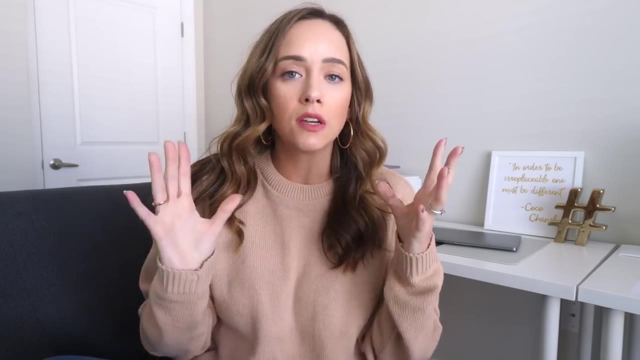 robot Sad times man, I'm still human, I'm still just mere mortal. Exhausting. And when I go back and I look at so many comments from this community, so many conversations I've had with clients so many times in 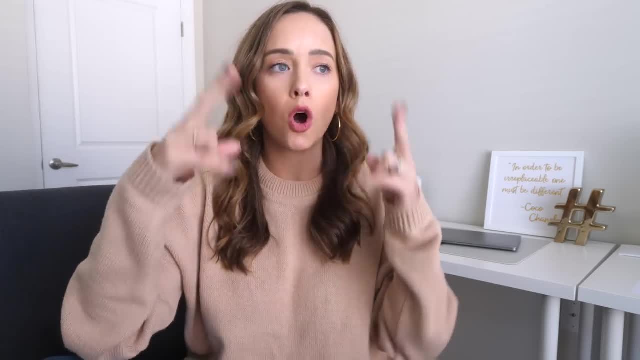 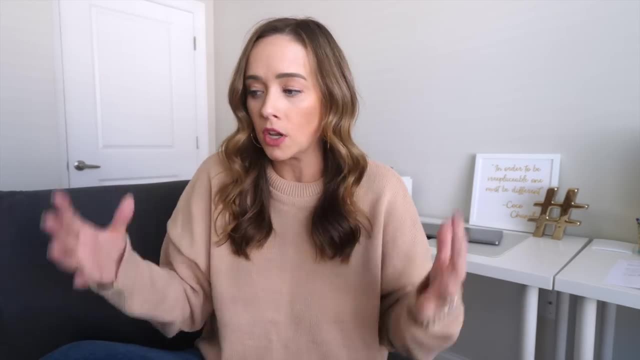 my life, where this dynamic of being a parent doesn't always compute When someone's saying, yeah, but how do you get things done when you have to deal with somebody else's life and taking care of them, and all these different dynamics and all these different things- your time batching thing. 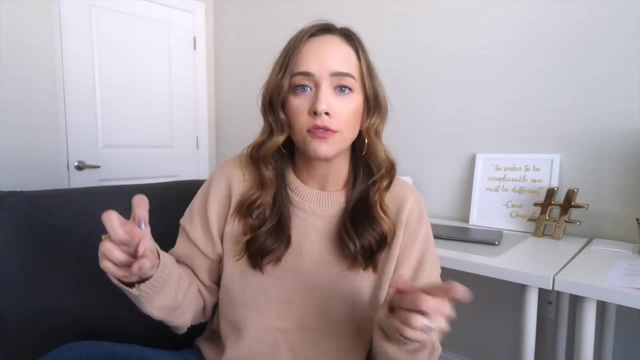 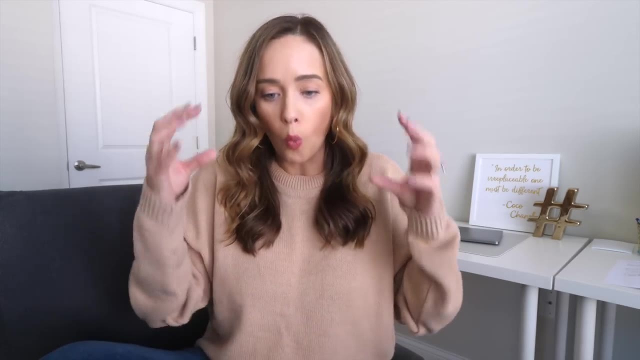 doesn't work for me. I didn't plan enough time. accordingly, I ran out of time. There's not enough time in the world. There's always so many stories around it, And I'm starting to understand why they are not just stories we tell ourself, but they're stories that are kind of true. 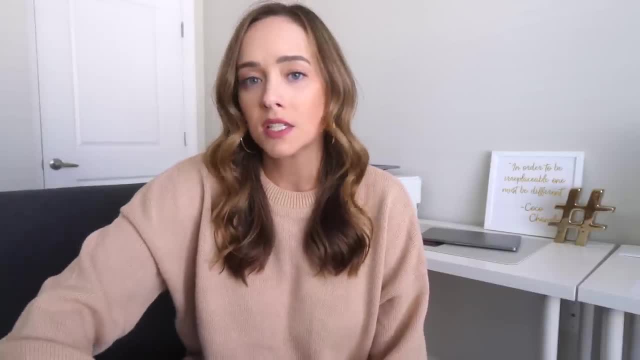 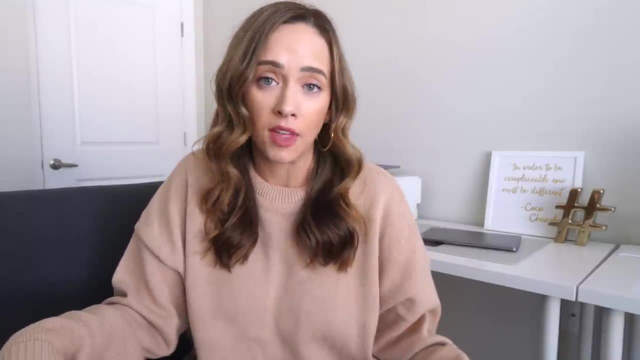 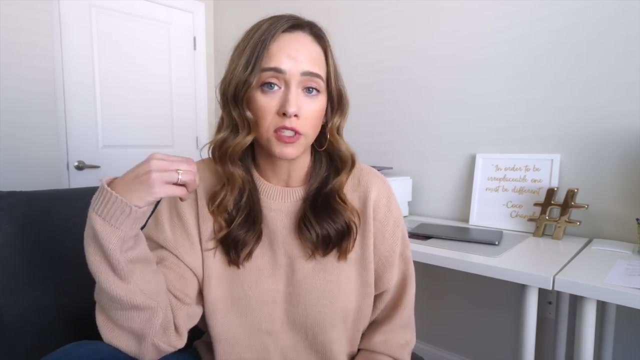 And it's because if we do not incorporate the help of others, it is increasingly harder to follow any of that advice, Mostly because you really cannot focus in general when there's another human involved. Now, the advice that you can't have a morning routine with kids, I still don't. 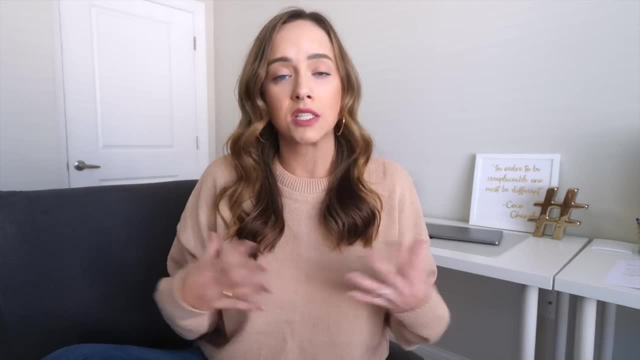 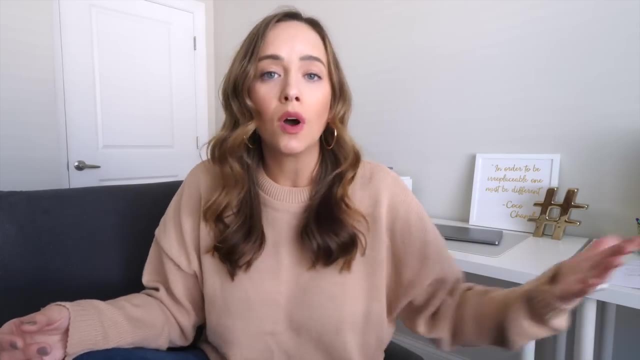 necessarily believe, because I think you can incorporate them into the process and your morning routine just evolves with you. My morning routine has evolved. I still do a lot of the same things, but I've got a kid next to me while I'm doing. 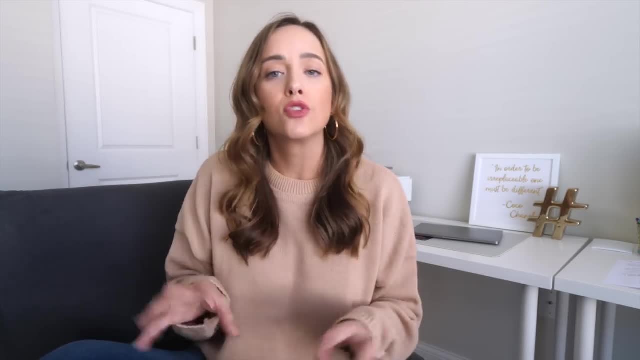 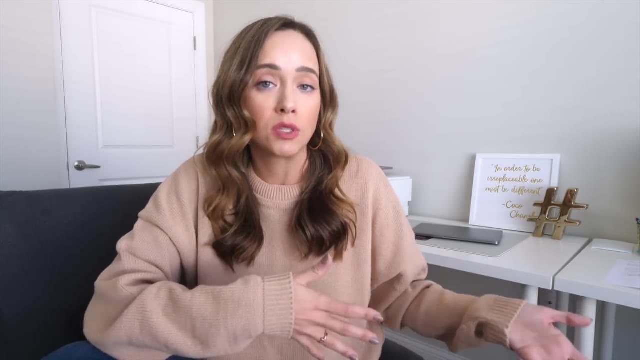 them, and she's entertaining herself in another way, And she's six months old now, So there are some things she can do to entertain herself now that she's awake more parts of the day than she used to be, But there are still things that are very important to me that I still stick to, And 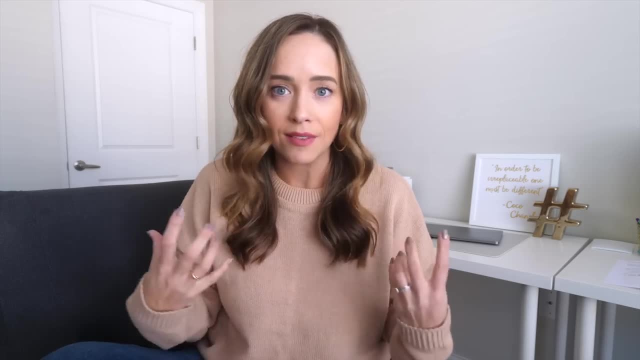 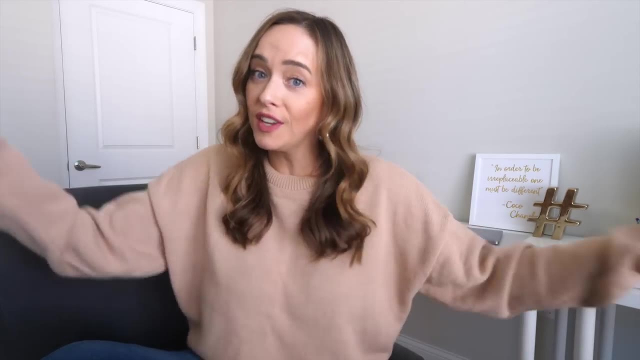 because of that focus and because of that need, I can make that happen. But if I need to do something like work or an appointment or a phone call or shooting, I can't do that. I can't do that. I can't do that. I'm shooting a video and I really need a kid not to be pulling on my hair and messing up my 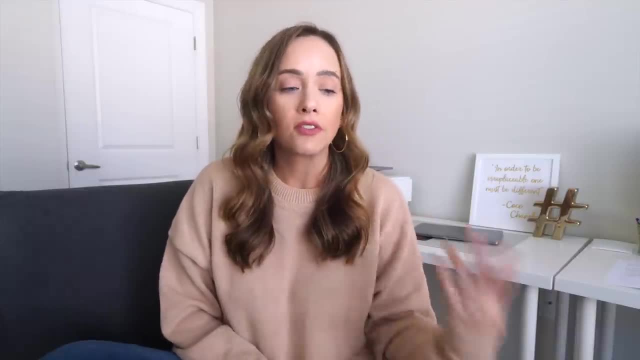 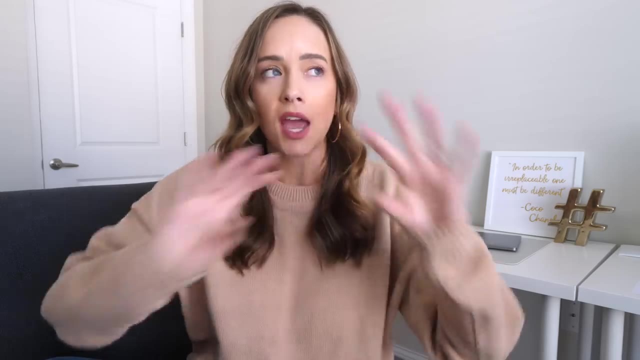 face and my makeup. I need to just be alone. for this I've got to incorporate help, And so I look back at all those comments and I look back at all of those struggles and I feel like the missing component for absolutely everyone, especially for parents, when it comes to time management. 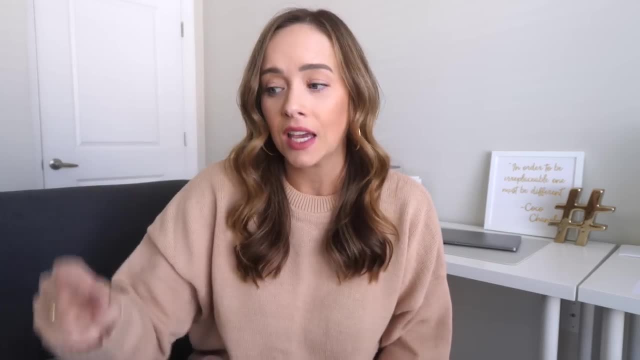 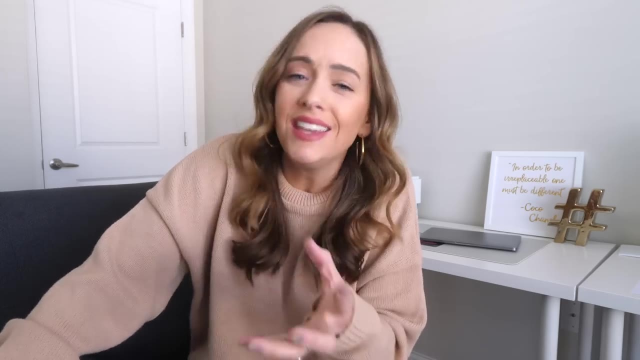 and hacking our way to success is asking for what you need when you need it, even if you don't even need it, Like you don't need somebody to do something for you. You don't need somebody to do something for you, But it would be nice if they did, because it would take that monkey off your 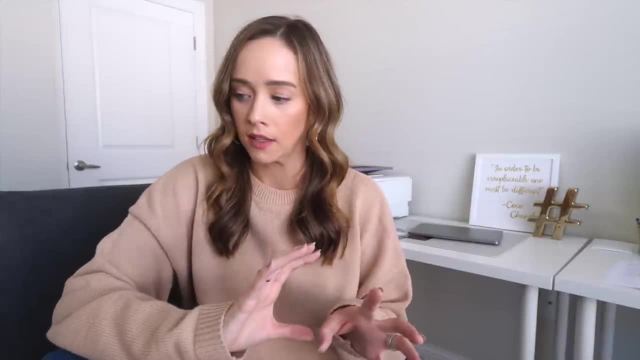 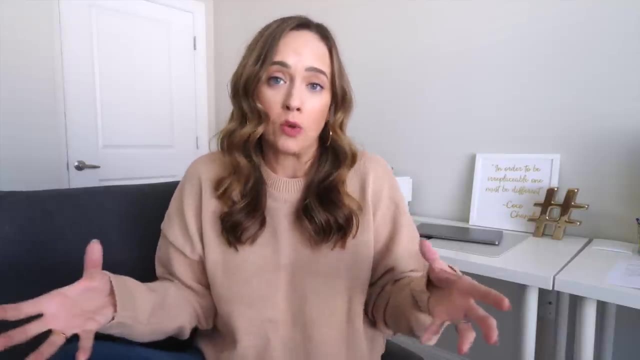 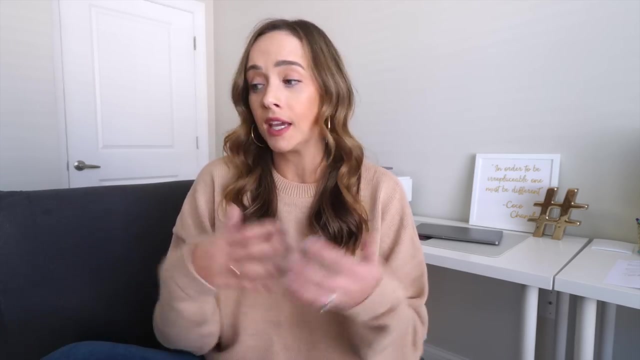 back. I think I'm just finally realizing the pinnacle of what it means to be superwoman- Like many women that are ambitious feel like they need to be- And that is taking care of their kids and doing all the things and working and showing their kids that they can accomplish so much if they try. 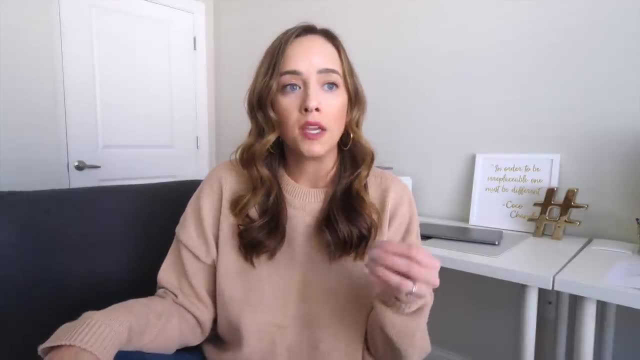 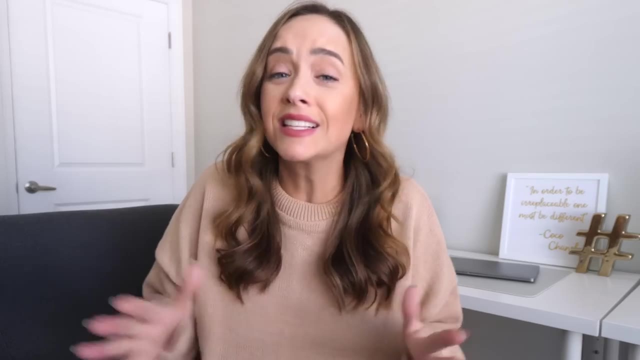 hard and work hard like mom, And yet we still are so strong To a fault. So I know this was kind of like time management tips for parents, but I am six months in guys, So I have absolutely zero intention of telling you how to hack your time as a parent. 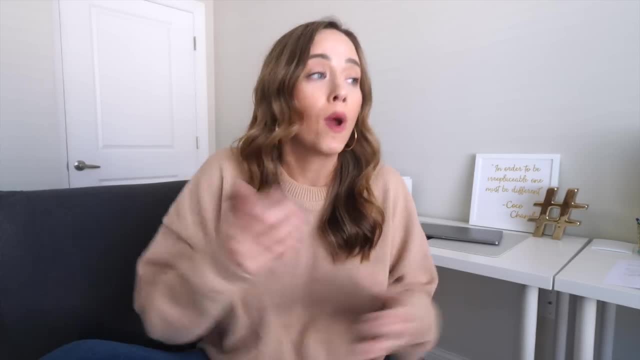 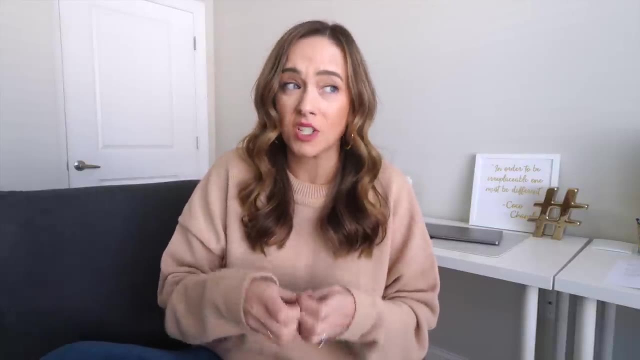 but this is what I have learned so far. What I've also learned is when I batched only three hours this afternoon to get the core of my work done, which is literally all I could do today. This is all I could do it, Not because I don't have more to do, not because I don't need more. 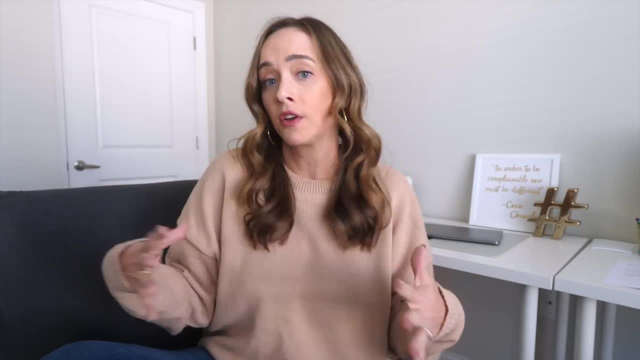 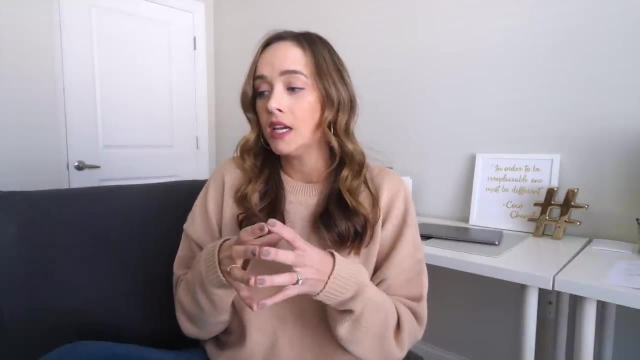 time, And I know a lot of people need eight hours, They need 10 hours and they need to figure out their lives accordingly. I just needed three today, which felt like an insane feat, And by taking that three hours I was able to get a lot more. 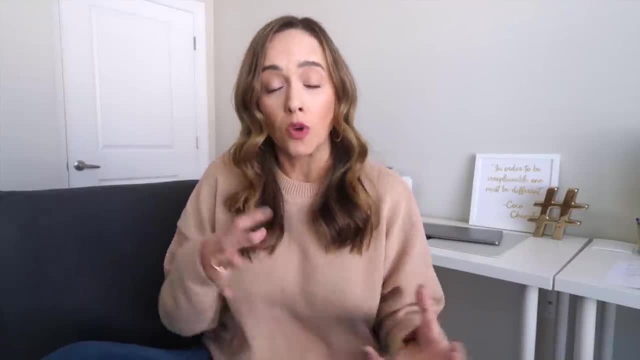 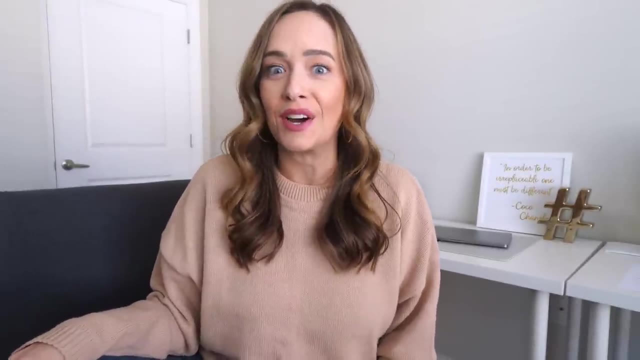 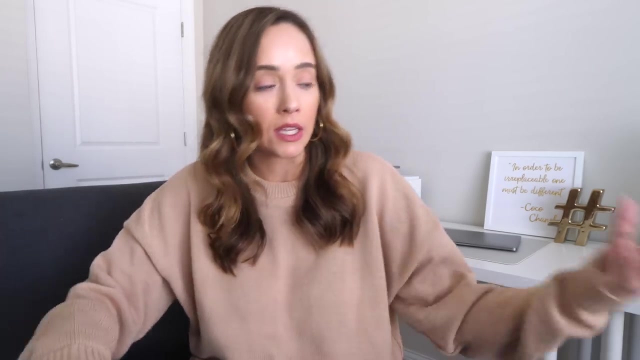 done in that space and time because it was batched with only certain types of tasks. and I have to do it. It's got to happen because otherwise it doesn't happen. And when I leave here and then I walk in the door where my kid is, where my husband is, where my family is, And you know that feeling when you 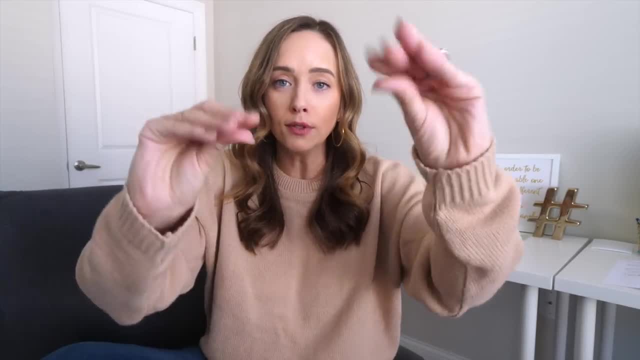 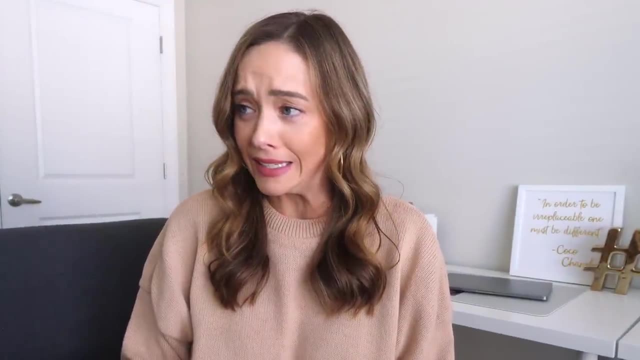 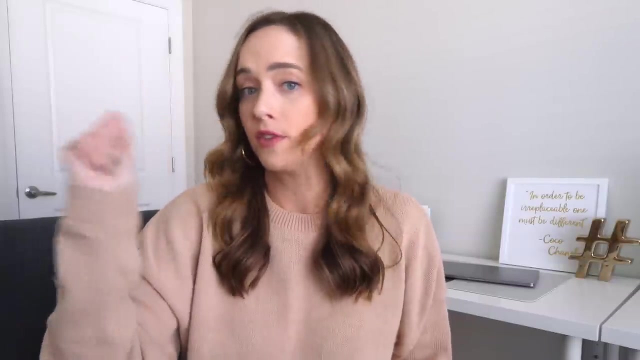 walk in the door. you walk in the door and everyone's like: can I take my shoes off Just one moment please? And it's nothing against them. It's just that that dynamic has now changed and the whole got to be on for everyone else. Switch has flipped again. Woo, That switch is getting. 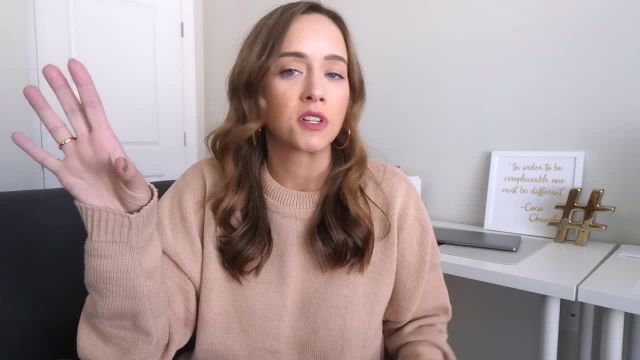 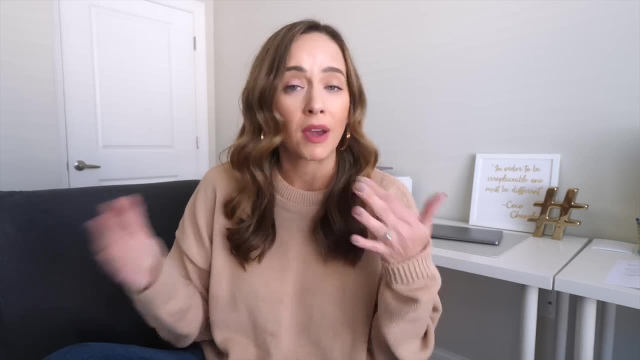 flipped all of the time for me. I have so many other personal reasons. There's just stuff going on. I'm currently in Columbus, I live in Palm beach, Florida, and we've been kind of going back and forth between Columbus and Connecticut just visiting. 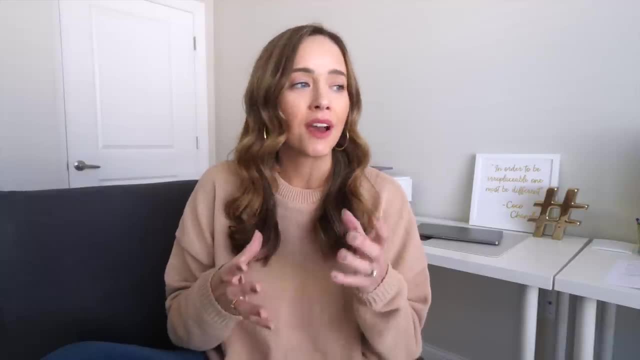 family And it's such a great time to be doing that because Bianca's growing up so much right now. The it is. you know how they say, you'll know when it's your kid, you know when it's your. 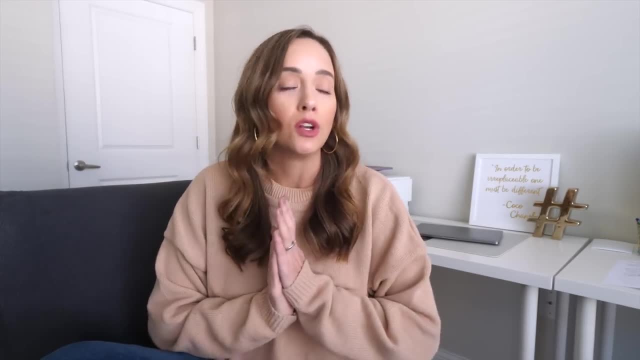 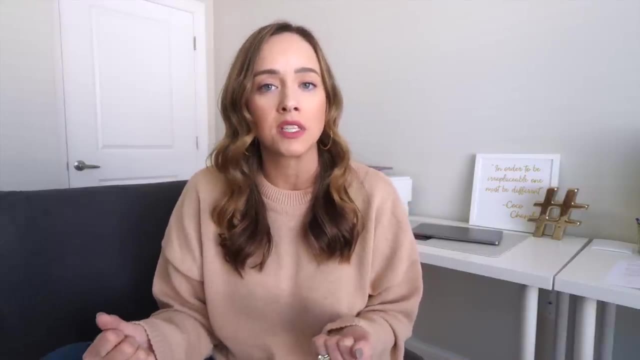 kid like to think about how different she is between you know three months ago And now is just mind boggling where I could never really compute that Someone else's kid, Cause you see it every time she wakes up from a nap, Every time there's. 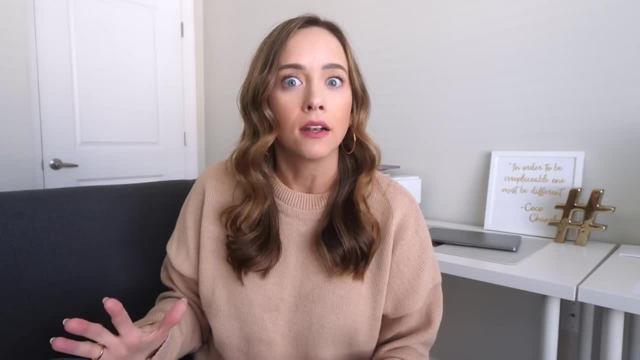 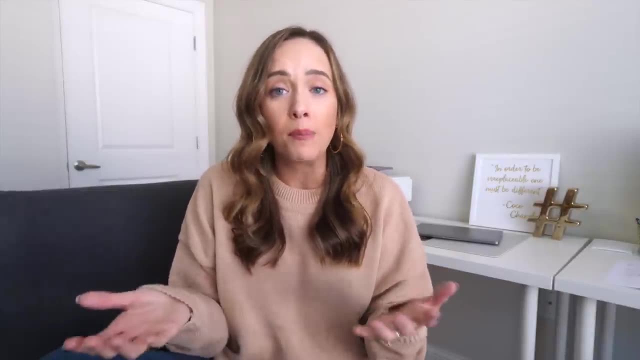 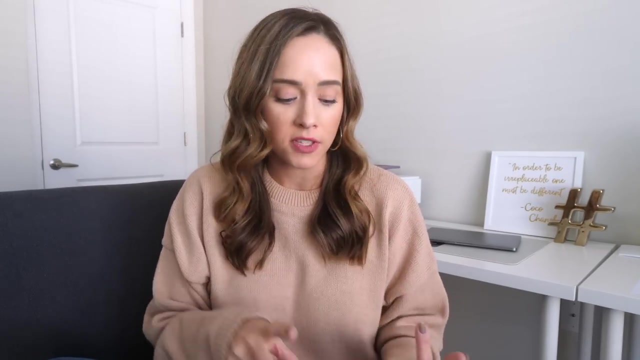 something going on. it's like what you just grew up again You again like what It's crazy. So it's really fun to be around family while they're seeing that all happen, because I feel like I'm making it more real for them. Um, so, you know we're dealing with that. I'm not in my home office. 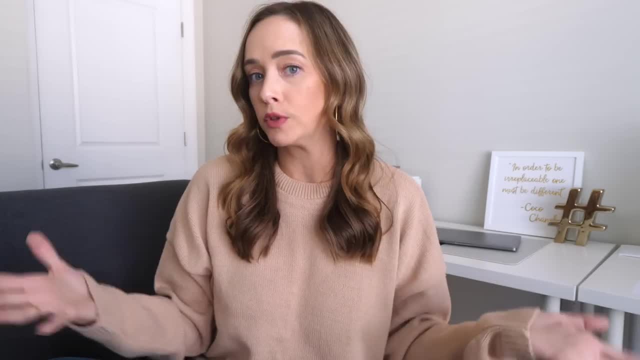 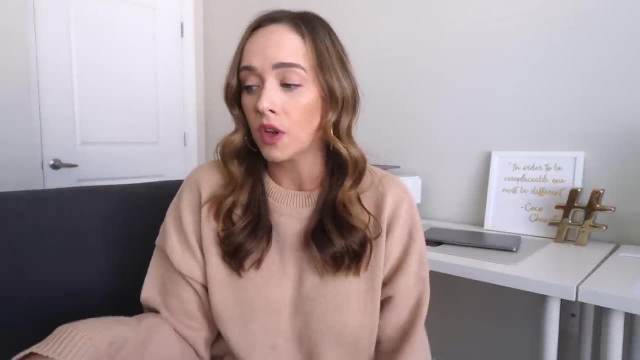 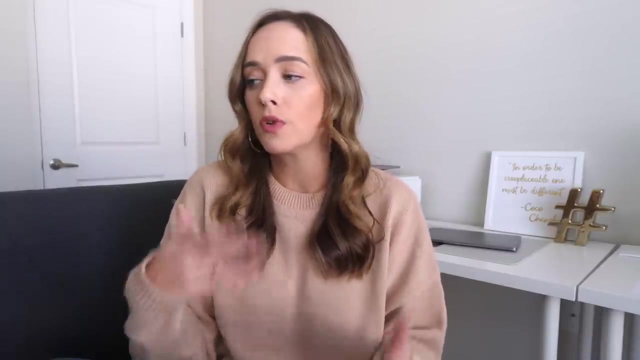 I'm not in my perfect little environment where I can do my routines accordingly. Bianca doesn't even really know where home is. She's too young. We keep moving her around and doing all this travel and stuff, which again I think is great, but also on the routine side of things tends to be challenging. So you throw all. 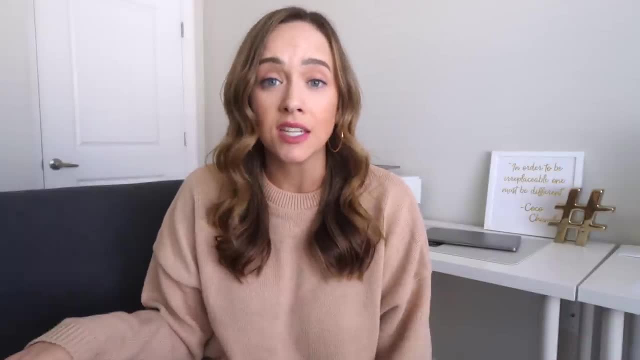 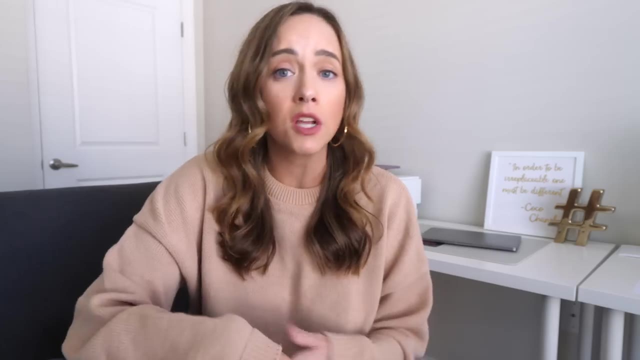 of this into it. This is what I have learned in terms of getting things done. I'm still running a business. I'm still trying to keep things going. I'm keeping the lights on. I'm making sure videos get done. I'm doing all these projects. We're working with clients. I've 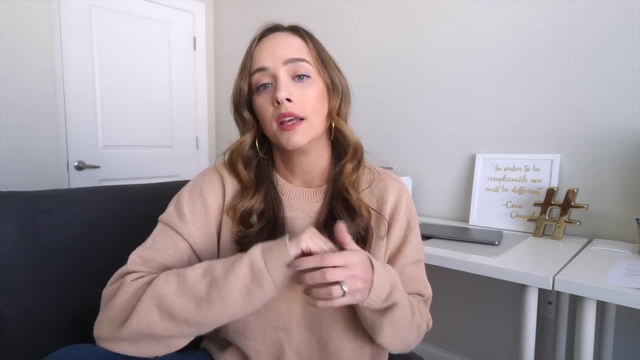 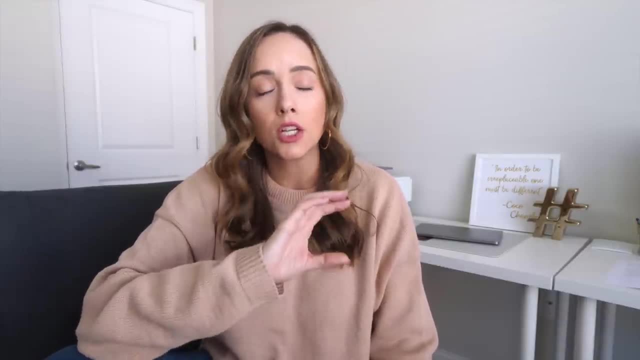 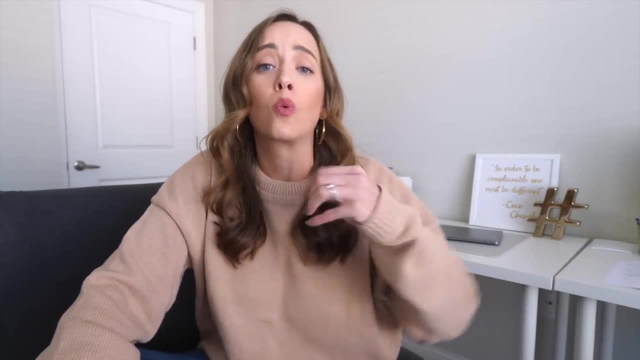 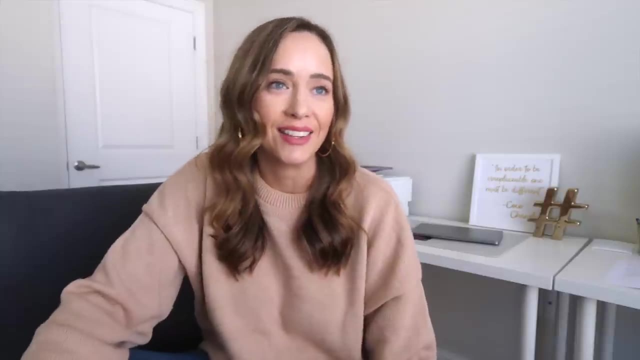 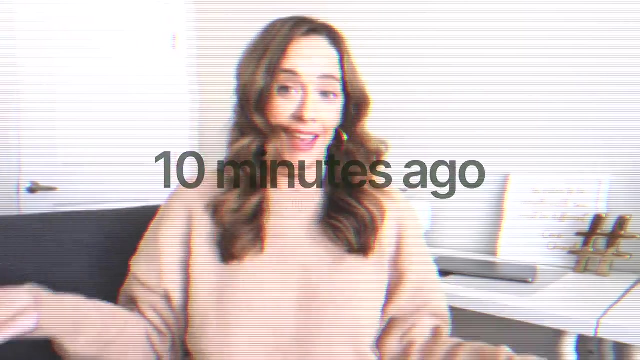 I have never said that it works for every single person, no matter what my advice has been in the last you know, whatever, Although I do feel like I probably kicked off the episode saying that my tips do work for pretty much everyone. I know anybody, literally anybody, but they only work. 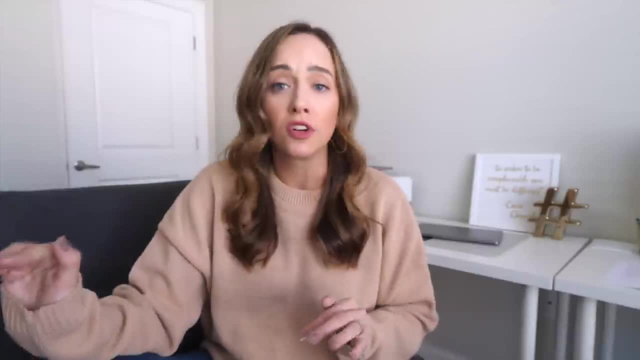 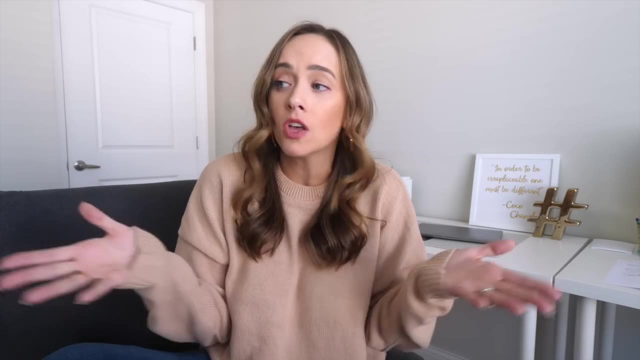 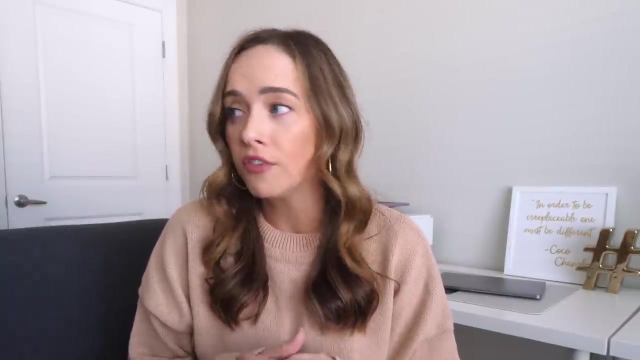 for anyone at all, If they, if it fits the mold of your life or not, if you believe wholeheartedly at giving it a good try and focusing on it. And that's all I know, That's what I know, And I literally can't do it alone And never, ever, ever in my life have I encountered something. 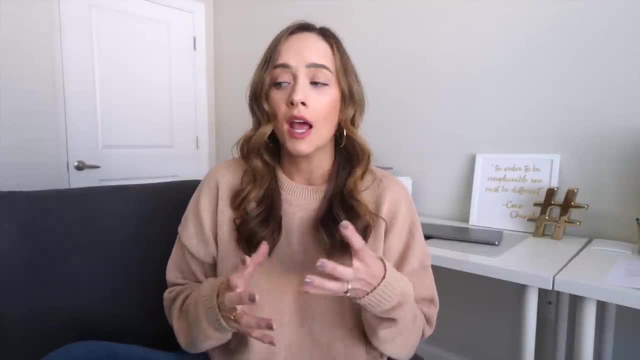 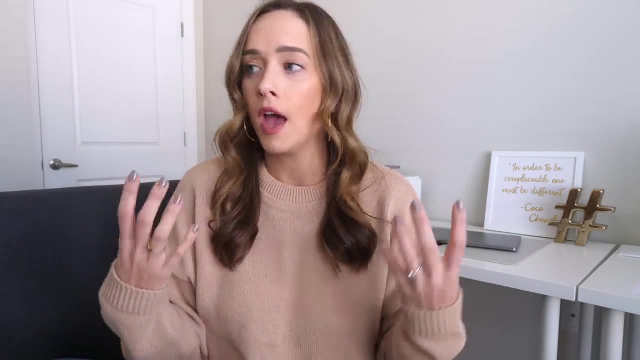 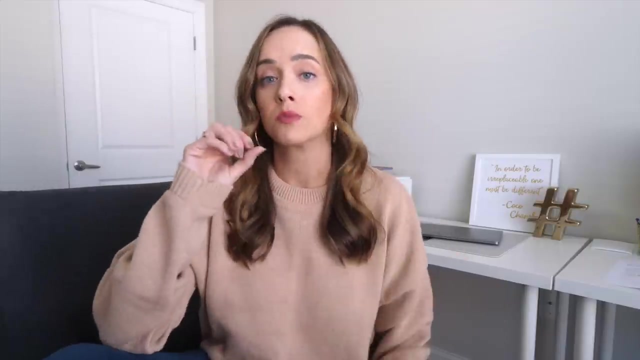 that I need to do, that. I want to do that. that brings me a lot of identity and self-love and importance and drive and passion and ambition for me. without needing help, Like it just blows my mind, I literally can't do what I love right now without asking. 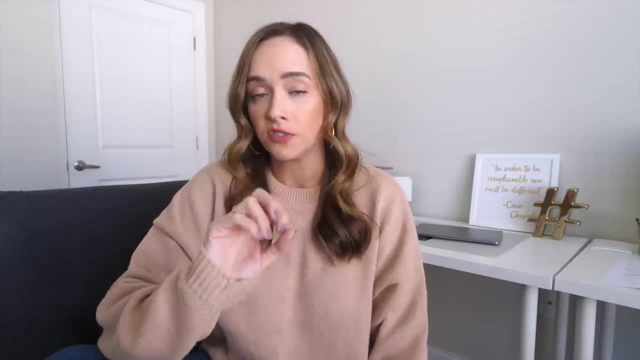 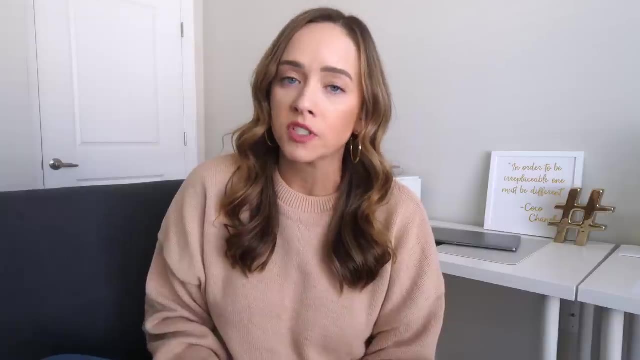 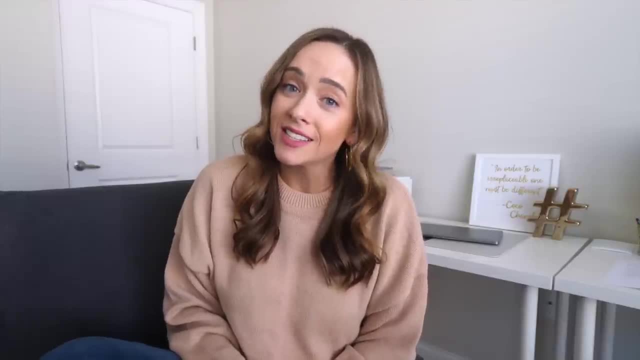 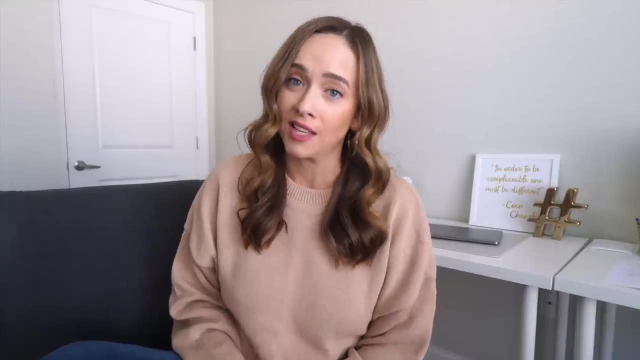 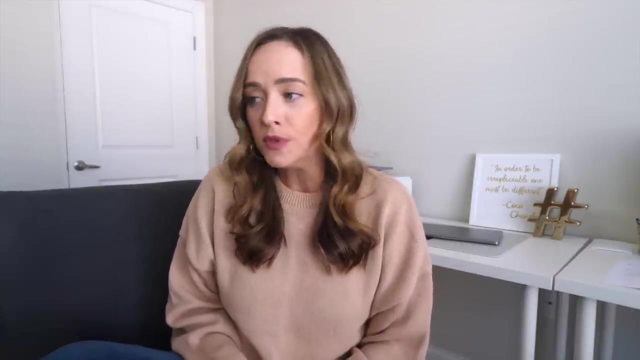 the universe is saying: ladybug, you should have learned this long time ago, So now we're cramming it down your throat. Okay, And her name is Bianca. Bianca is teaching you You need to ask for help, So there is no hack. It's hard, You have to communicate with people. It's hard, but you. 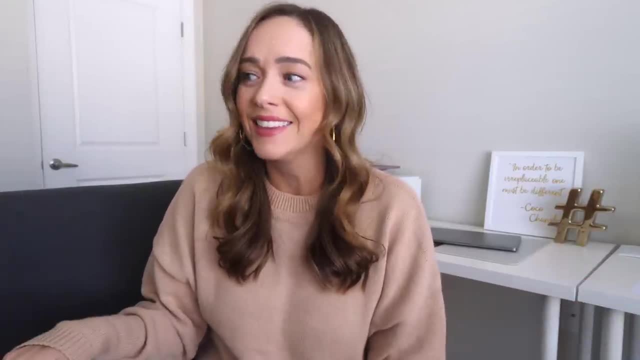 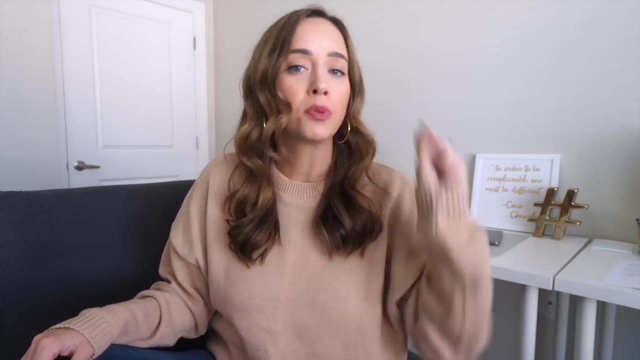 know what. It just sucks. That is the answer to everything. The answer to everything is good communication, like really rock solid, effective communication. not I need to put you in your place communication. not I'm going to tell you what I need and I don't.